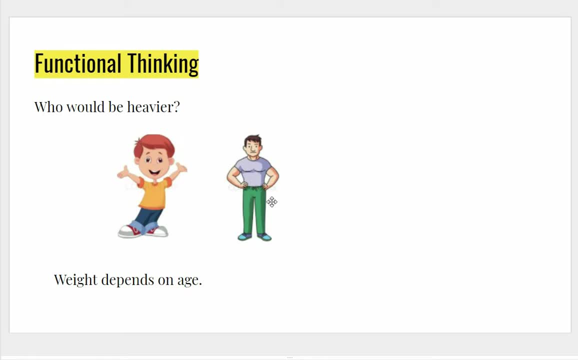 a child and here is an adult man, well built, And you don't have to weigh them to tell me that this man is heavier than the child. So you'd say that weight depends on age. That's why the person who is younger is likely to be lighter. 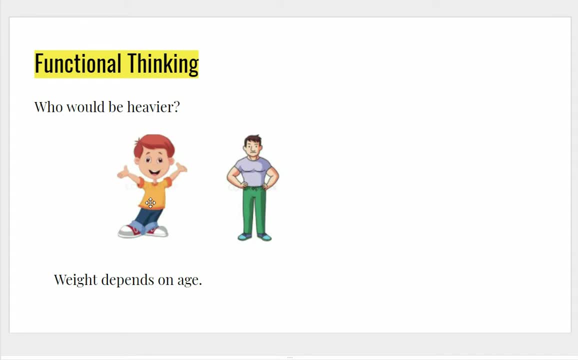 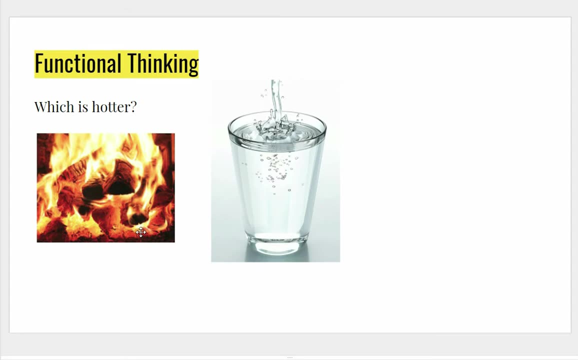 Not always true, but in this picture that's the functional thing that you can guess. Another example is a child which is hotter. You have two pictures: This is fire logs burning and here is a glass with cool water. So looking at the picture, you can say that. 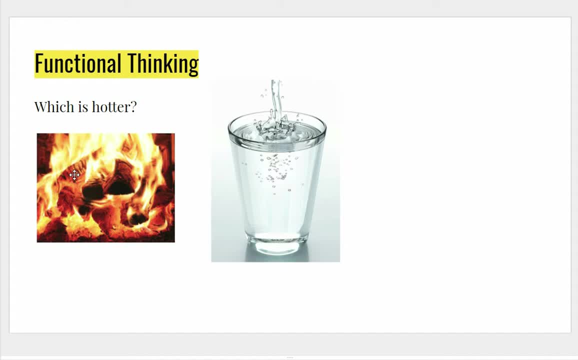 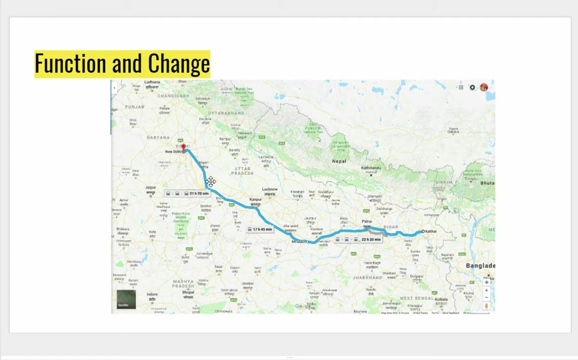 the one on the left would be hotter. So we are trained to always guess by looking at what we have, and in calculus we call that function. So now coming to the next step. So now coming to function and change. So the diagram you have here, let 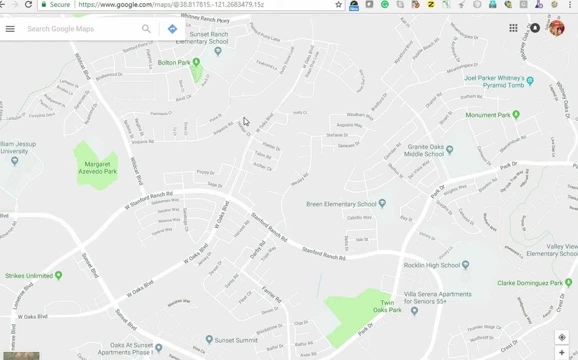 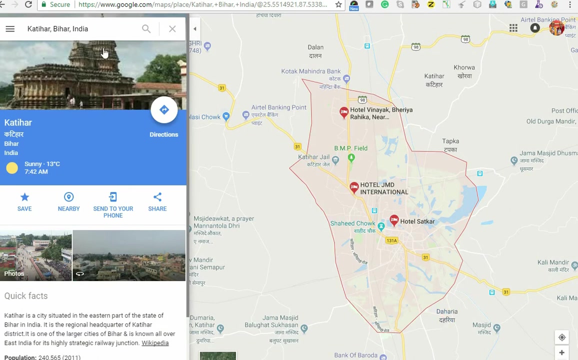 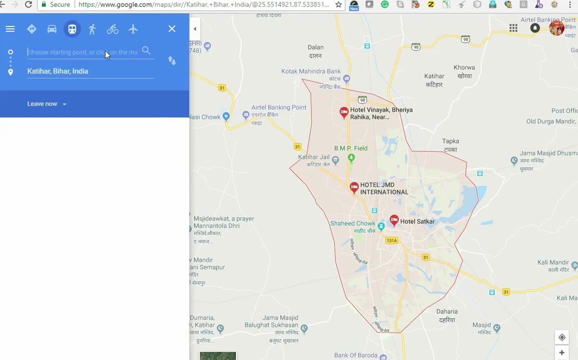 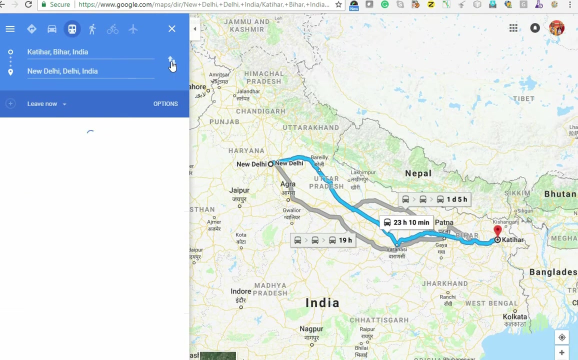 me go to Google map. So here is Google map, and at first I choose my place of birth, Kati Har. This is the nice view of the place And and I look for directions to Delhi. let me switch the locations from Katihar to. 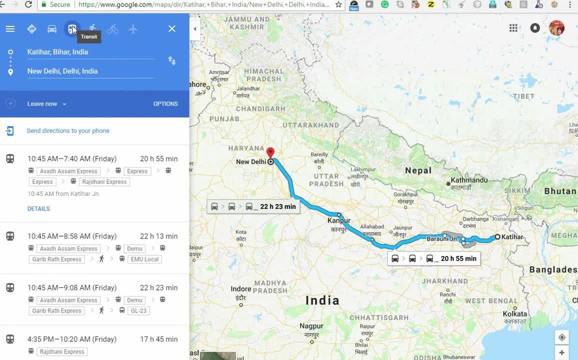 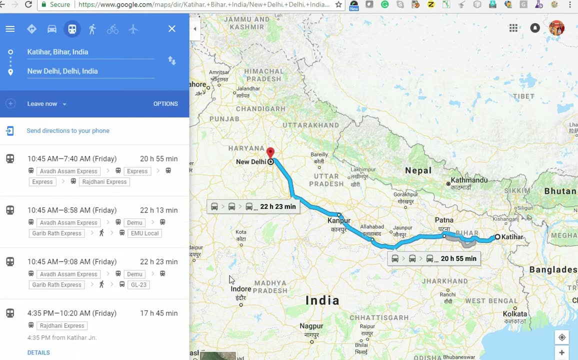 New Delhi and I take transit train. so on Friday we have Rajdhani and it gets reaches Delhi in 17 hours 45 minutes and it takes this route or route. so here is Kanpur and New Delhi and train moves along this route. so, as I was saying that, 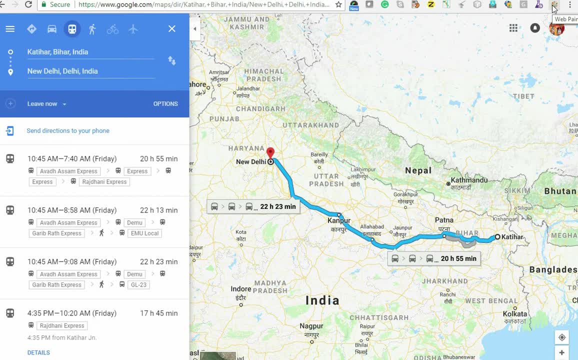 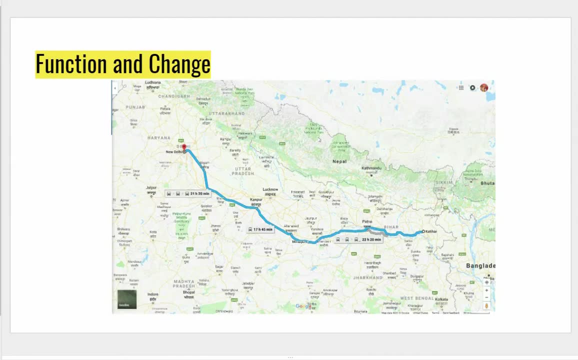 calculus is about movement, so now we will put this data in a table and see what it looks like. all right, so we are back to this spreadsheet. this picture of the route Rajdhani Express takes from Katihar to Delhi. so I put this in this data format and 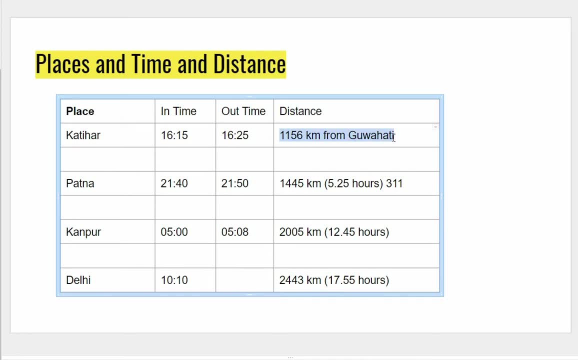 let me change this. so let's start from Katihar at 0 kilometers and but now would be 200, 89 kilometers, Kanpur would be 849 kilometers and Delhi is one to eight or seven kilometers kilometers. So the time it takes 5.25 hours to reach from Katihar to Patna. It 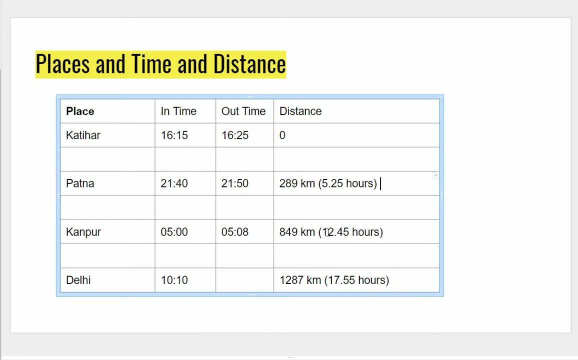 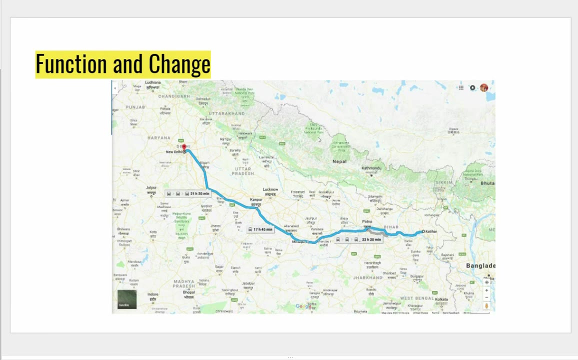 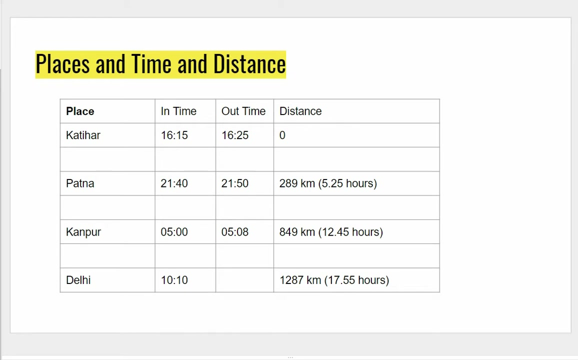 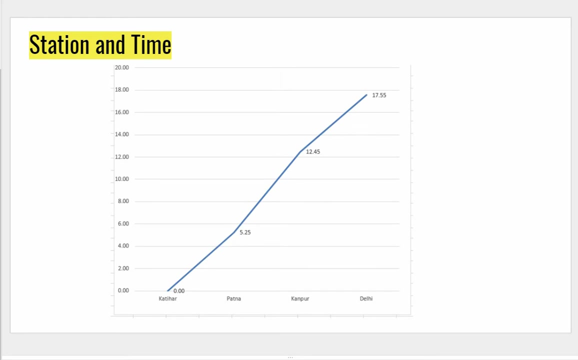 takes around 12-13 hours to reach Kanpur and around 18 hours to reach Delhi. So this data and you can talk to your kid about this picture and what the data looks like in this format. So now we will draw this plot. So what we have here on 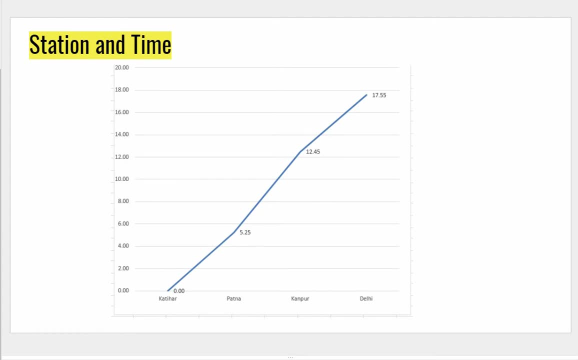 this map now I can draw on this all right. so this is my location and this is the time in hours. So here we have zero, two, four, six, eight, ten, twelve hours like that. So We said we are taking Katiharada starting point, so over here, in 5.25 hours it reached Patna, and this is Kanpur and this is Delhi. 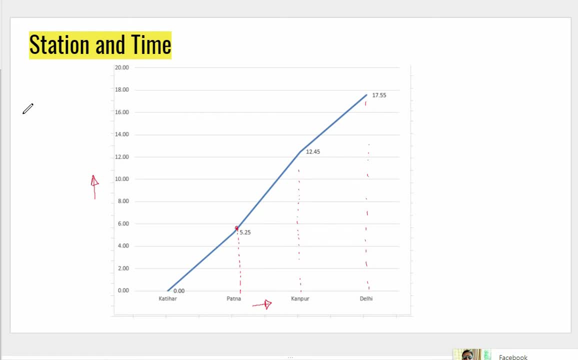 So when we moved from Katiharada to Patna, the time elapsed is 5.25 hours. When we move from Katiharada to Kanpur, time elapsed is 2.45.. So if I put an arrow here, so time is moving in this. 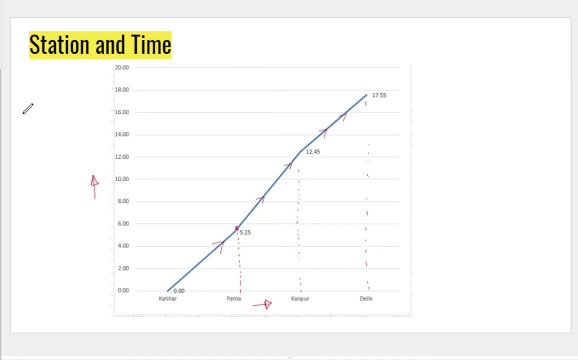 So this is the station and time plot. I had learned about plotting when I was like in 8th or 9th grade And I tried this with a couple of kids recently and they were able to intuitively grasp this concept of plotting and the concept of change. 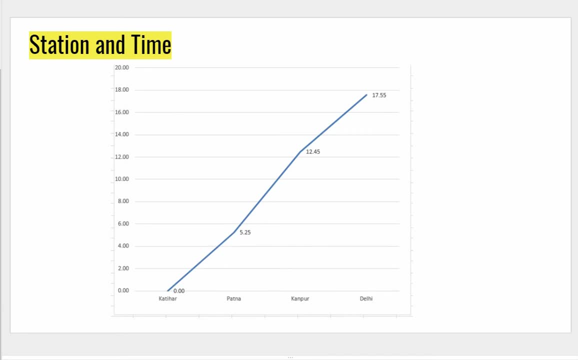 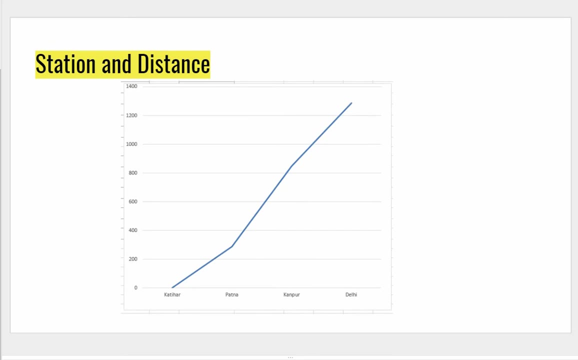 Now the Next thing Is plotting of station and distance. So Let me And restart. So here, we took Katiharada to be the starting point. Patna is here And We had Is 289 kilometers. 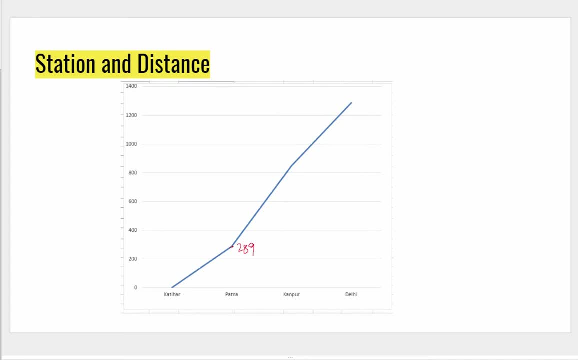 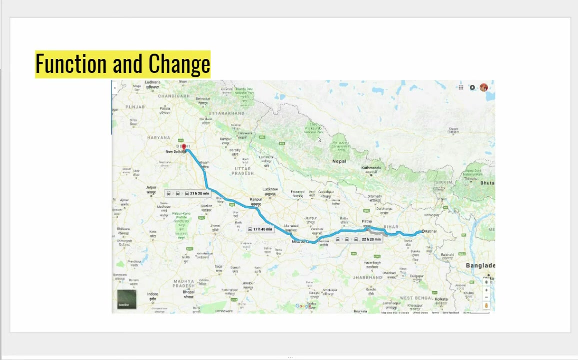 Kanpur is here 849 kilometers And Delhi is here 1287.. Now we go back to the map. we go back to the map and choose a spot. So so here is Allahabad. So here is Allahabad. 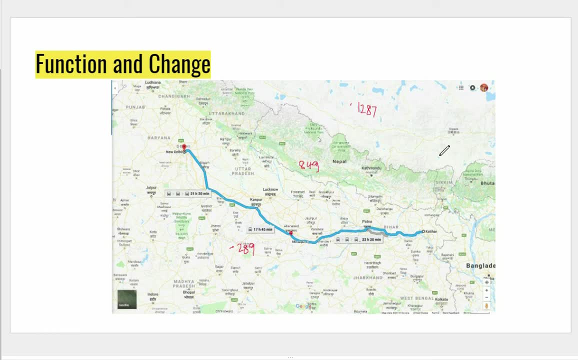 So here is Allahabad, And Allahabad is between Patna and Kanpur. So Allahabad a railway station is between Patna and Kanpur. So Allahabad a railway station is between Patna and Kanpur Now. 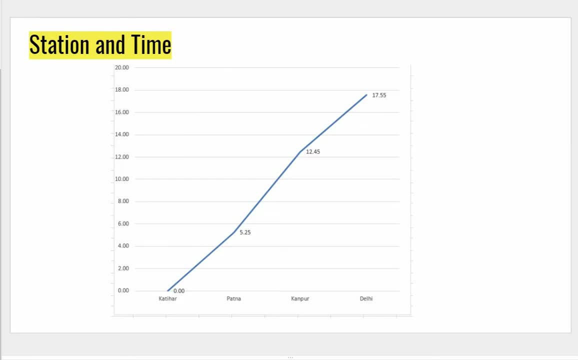 I ask your child this question- That Usually we say that we are on the reservation. Yes, We are on the reservation. Now If what is written in the计 Rocket, The newspaper When we write Is there, if or when there is. 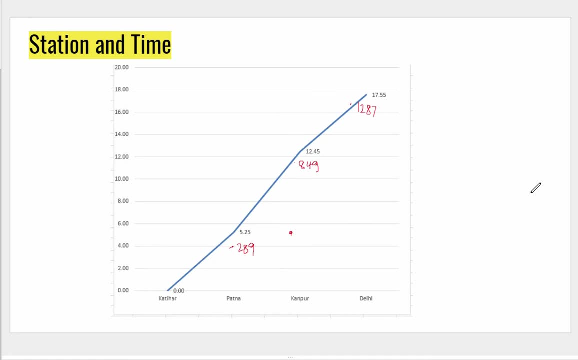 If you go back- So he was right here- I will hang island, Because that's where we are over here In in a wonderful way. It's not wrong. I do see That there is an island there, Oh, oh. 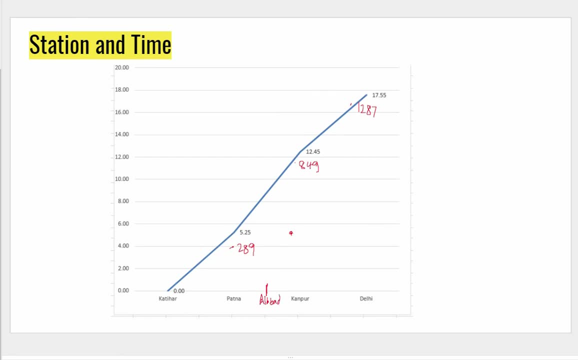 OK, Allahabad, all right. so now I ask you to guess that, if the train reached, but now in 5.25 hours, and Kanpur at in 12.45 hours, where the time at Allahabad will lie, so we can guess that if it is somewhere here. 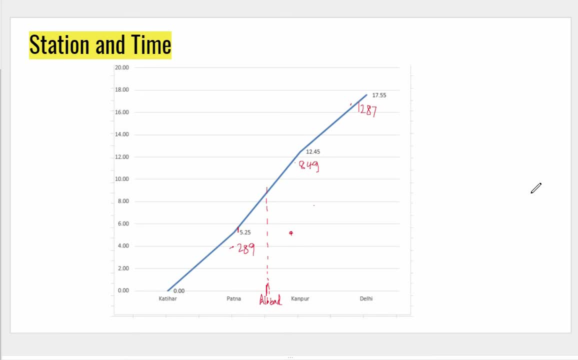 if it is somewhere here, then the time should be between 5.25 and 12.45. so if I write here, time at Allahabad will be between 5.25 hours and 12.45 hours. so this is a guess, because we know that Allahabad comes after. 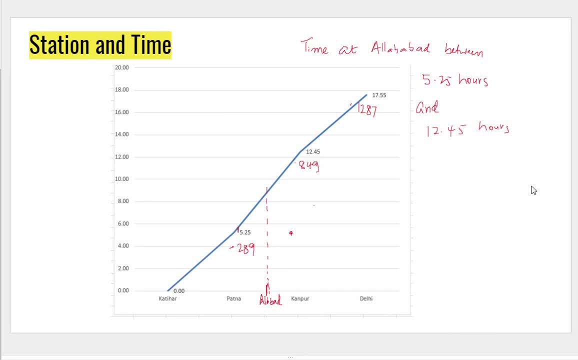 Patna and before Kanpur, the time the train it takes to reach Allahabad will be that after the time it took to reach Patna and before the time it took to reach Allahabad, Kanpur. now we guess the distance if Patna is 289 kilometers from Katihar and 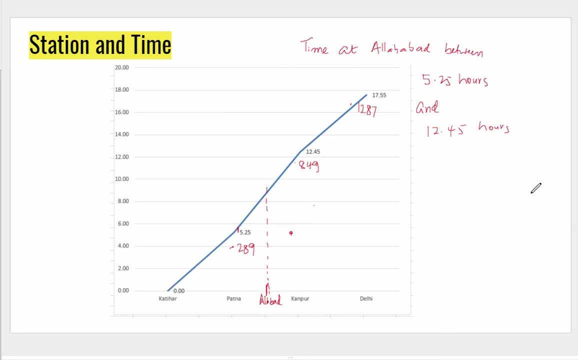 Kanpur is 849 kilometers from Katihar. so the distance same thing. distance will be between. distance will be between 289 kilometers and 849 kilometers. so we can safely say that Allahabad cannot be move less than 289 kilometers from Katihar or it can be greater than 839. 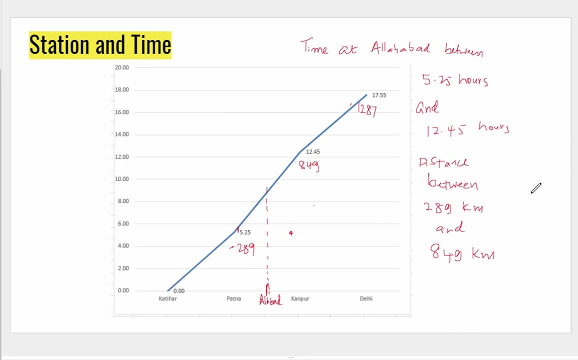 kilometers, 49 kilometers from Katihar. It has to be in between. Now we'll have questions like how we can guess how long it takes from to reach from Katihar to to Allahabad, or from Patna to Allahabad, and what would be the distance of Allahabad from. 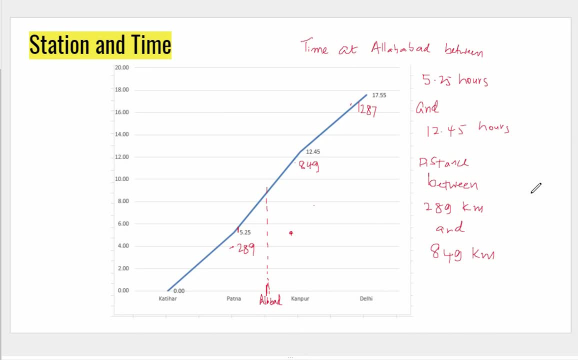 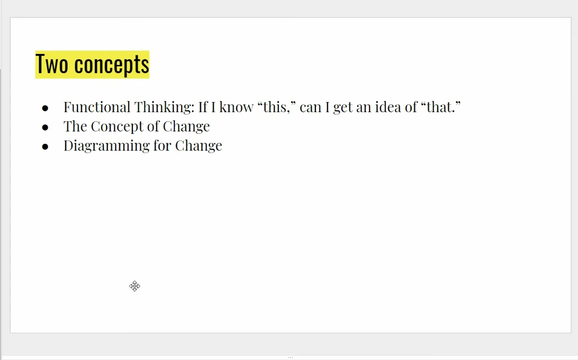 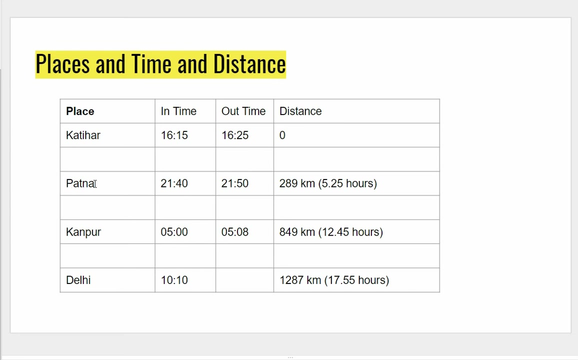 Katihar to Allahabad. So these are the questions that we will handle in the next tutorial on this topic. So, revising this, what we did, we looked at functional thinking and the functional thinking was that the distance of a station from Katihar. if we know the time, we can guess the distance. 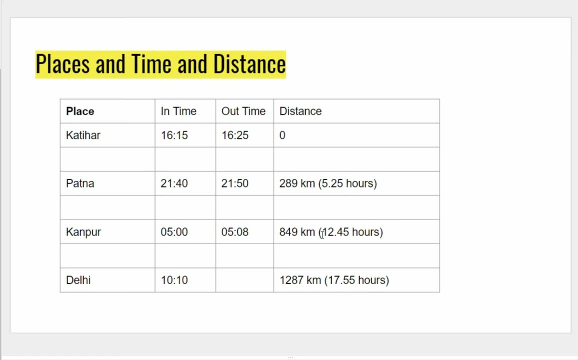 or if we know the time, we can guess the distance. sorry, I repeat it: if we know the distance, we can guess the time. if we know the time, we can guess the distance. that's the function, and here we learned to plot. so this plot is by hours. 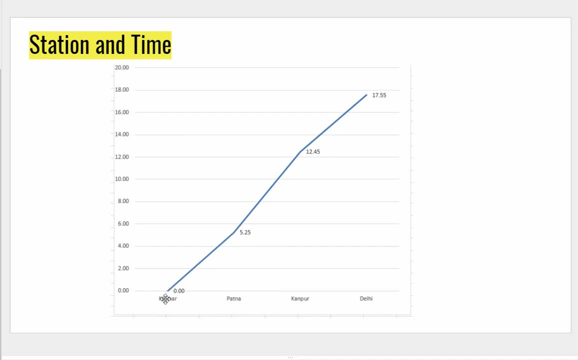 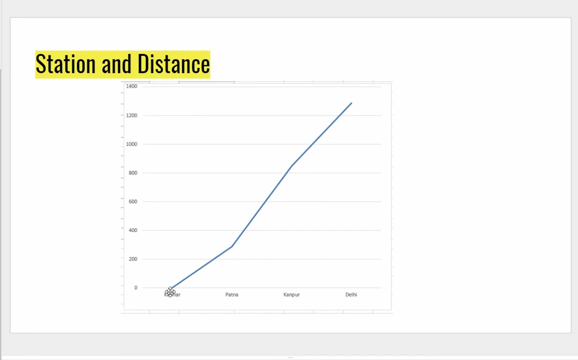 and location. so as we move from Katihar towards Delhi, we move in time and distance. as we move from station to station, we gain distance. This is the way to learn to plot, and in the next tutorial we'll learn about how to calculate the rate of.